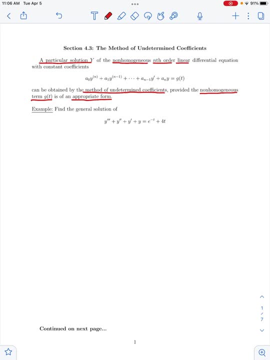 And the way that it works is by substituting that particular solution into our non-homogeneous equation. So let's look at some examples of how this will work for higher-order equations. In this first example, we are asked to find the general solution of this third-order linear. 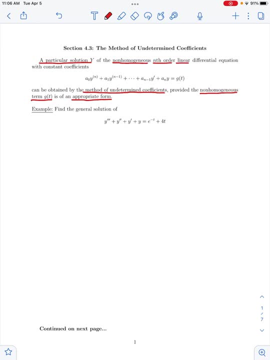 non-homogeneous equation with constant coefficients. So we know our first step to solve a non-homogeneous equation. The first step is to consider the homogeneous equation: y, triple prime plus y, double prime plus y. prime plus y is equal to zero And to solve this we could look for solutions of the form. 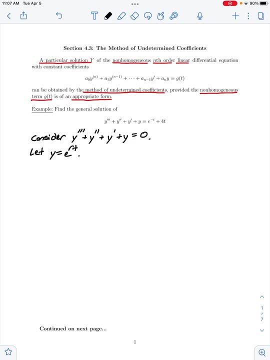 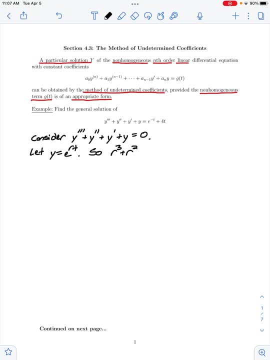 So we can look for solutions of the form: y equals e to the r times t power, which means that r has to satisfy the character of t. R cubed plus R squared plus R plus one is equal to zero, And I could factor this by first factoring out an R squared from the first two terms. 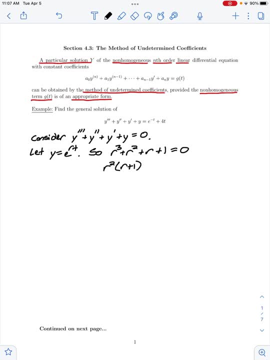 which would leave me with an R plus one, And then I have another R plus one for my last equation: two terms. So if I factor out the common factor r plus 1, I'm left with r squared plus 1 is 0.. So it follows that my roots are: r equals negative 1 and plus or. 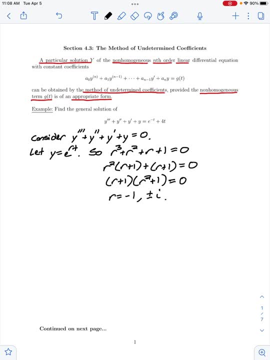 minus i. So for these roots, the general solution of the homogeneous equation, or homogeneous solution, would be c1 e to the negative, t plus c2 cosine t plus c3 sine t. And now our next step is to determine some particular solution Of the non-homogeneous equation And to determine the form of this particular solution. we're 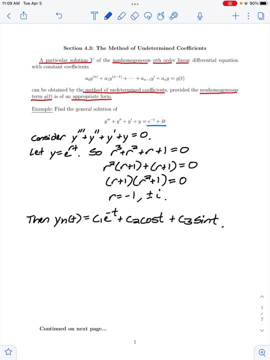 going to look at the form of this g of t function on the right-hand side of our equation And we see here that g of t is a constant times e to the negative t plus a first degree, or linear polynomial. So let's think, look for a particular solution of that same form, Capital y of t. We could take some constant. 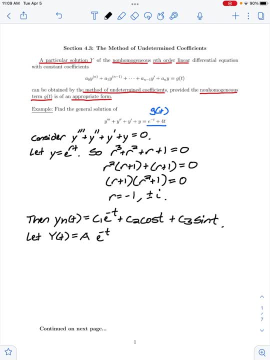 times e to the negative t. But we see that since r equals negative, 1 was a root of our characteristic equation that a constant multiple of e to the negative t is already part of the homogeneous solution. So for our particular solution, that first term we would consider would be a constant times. 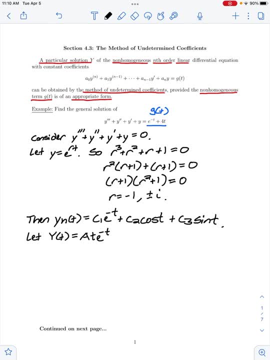 t e to the negative t. And then the last part of our g of t function was a first degree polynomial, So we could consider some general first degree or linear polynomial, Something of the form bt plus c. And now none of these terms are already part of the homogeneous solution, so this will be the correct form. 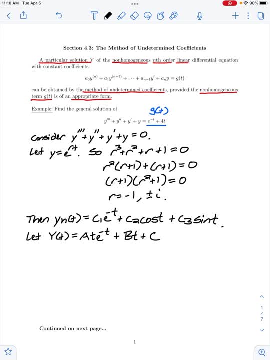 And to solve for a, b and c, we need to substitute into our non-homogeneous equation And, since this is third order, we're going to need to find our first three derivatives of this particular solution. So let's look at it. For capital Y prime, we have a times. 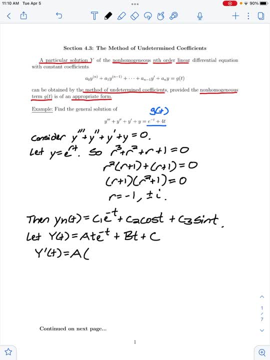 by the product and chain rules we get a: 1 minus t, e to the negative t plus b. Then for the second derivative we have a times a negative 1 minus 1, and then plus t all times: e to the negative t. 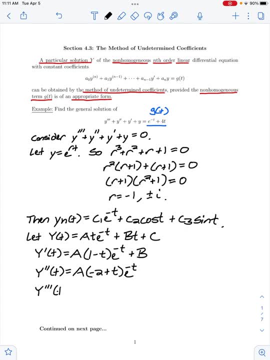 And then for the third derivative Y triple prime, we have a times by the product and chain rules we get a positive 1 plus 2, so 3, and then minus t e to the negative t. So let's take these expressions and substitute into our non-homogeneous equation and see what we 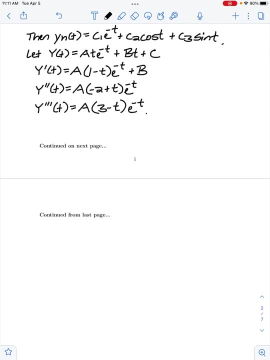 have. So here we are looking for Y triple prime plus Y, double prime plus Y prime plus Y, which has to equal our g of t function e to the negative t plus 4t. So substituting in these expressions that we found our third derivative is a times. 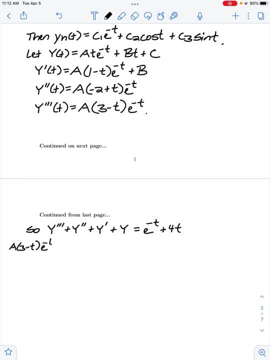 3 minus t e to the negative t, plus our second derivative, which was a times negative 2 plus t e to the negative t plus Y prime, which was a times 1 minus t e to the negative t plus b, and then plus Y, which was a times t e to the negative t. 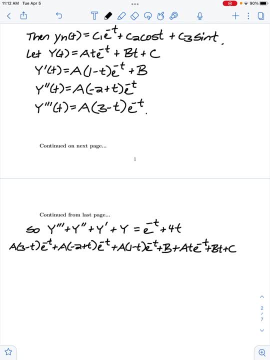 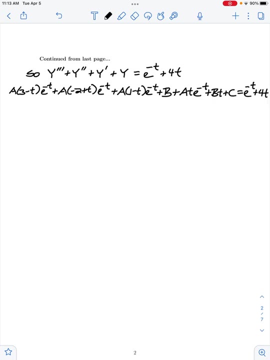 plus b times t plus c, and this still needs to equal e to the negative t plus 4t. So let's see what we get when we collect like terms here. Let me just go ahead and do this. Let me start by grouping all of the terms involving t times e to the negative t. 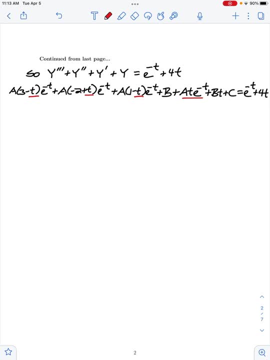 So, summing these terms, I have a negative a plus a minus, a plus a times t e to the negative t. So all of these terms cancel one another. We're left with zero. And now let me look at the terms that are just constants: times e to the. 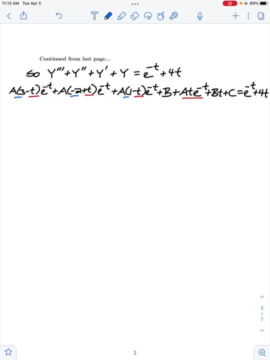 e to the negative t. So grouping these terms, we have 3a minus 2a plus a, which leaves us with 2a times e to the negative t. And then let me group all of my linear terms together. So here we have a b times t, and then a plus b plus c. 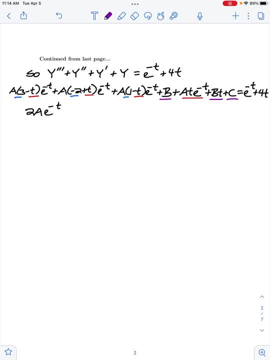 So here we have a b times t, and then a plus b plus c. So here we have a b times t and then a plus b plus c. So our coefficient of t is b, And then my constant coefficient was a b plus c. 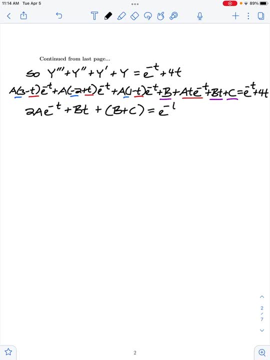 And this has to equal e to the negative t plus 4t, And this has to equal e to the negative t plus 4t. So, equating these coefficients, we find that 2a has to be 1.. So a is one half. 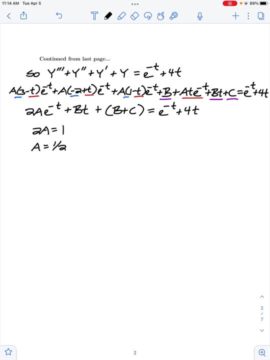 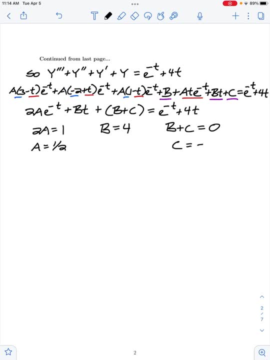 So c is the negative of b, which would be negative 4.. So substituting these constants back into the general form for our particular solution, we find the particular solution would be: A, which was 1 half T, e to the negative T. 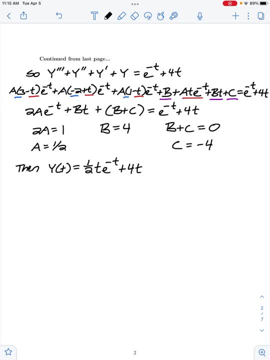 plus B, which was 4 times T plus C, which is negative 4.. And so, for our general solution of this non-homogeneous equation, we take the sum of our homogeneous solution, which was C1, e, to the negative T. 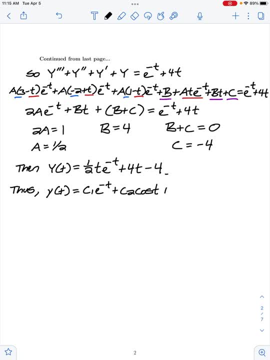 plus C2, cosine T plus C3, sine T, And then we add our particular solution, which is 1 half T e to the negative, T plus 4T minus 4.. So in this first example we see that the method of undetermined coefficients 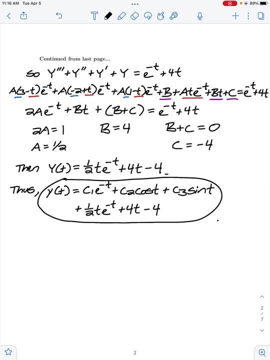 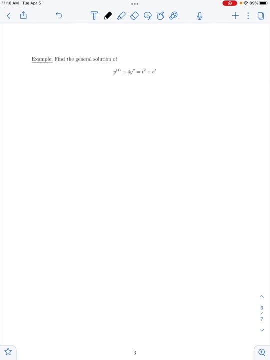 for higher-order linear equations works the exact same way as for second-order linear equations. We just have higher-order derivatives to evaluate. So let's look at another one. In this next example we have the same sort of problem. We are asked to find the solution of the non-homogeneous equation. 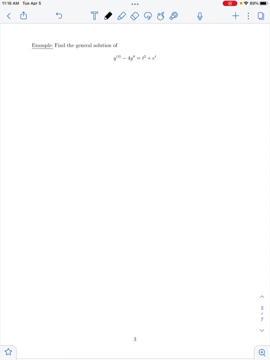 the general solution of this fourth-order linear non-homogeneous equation with constant coefficients. And so again, our first step is to consider the corresponding homogeneous equation. The fourth derivative of y minus 4y double prime is equal to 0.. And if we look for solutions of exponential form, 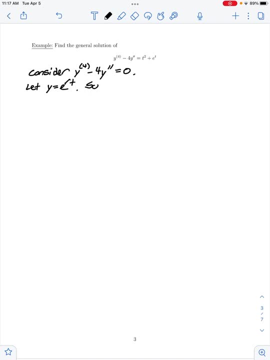 y equals e to the rt, then r must satisfy the characteristic equation. r to the fourth minus 4r squared is 0.. So if I factor out r squared, I'm left with r squared minus 4.. And then that quadratic can be factored as r plus 2 times rt. 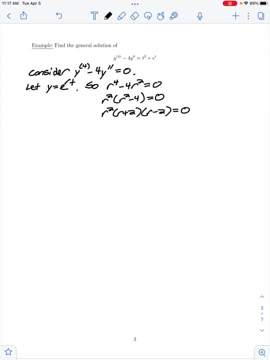 or minus 2.. So we find that we have roots of 0,, which has multiplicity 2,, negative 2, and positive 2.. So our homogeneous solution has the general form: c1 plus c2 times t plus c3 times t. 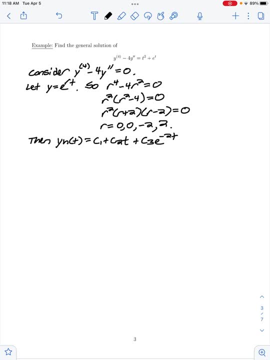 And then we have roots of 0,, which has multiplicity 2,, negative 2, and positive 2.. So our homogeneous solution has the general form: c1 plus c2 times t plus c3 times t, e to the negative 2t. 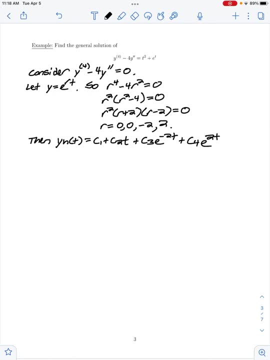 plus c4 e to the positive 2t, And now we need to find a particular solution. So when we look at this g of t function on the right-hand side of our equation, we see that it is the sum of a quadratic. 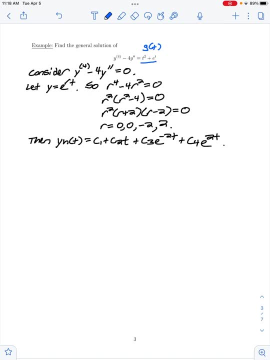 or a second-degree polynomial and a constant times e e to the t. So for our particular solution, we might start by considering something of the same form. Let's take a general quadratic at squared plus bt plus c, And then we could add a constant times e to the t. 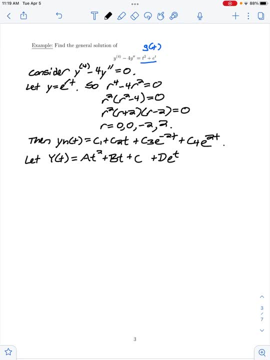 Now, when we compare this with our homogeneous solution, we see that both a constant and a constant times t are part of the homogeneous solution, because 0 was a double root of our characteristic equation. So the two terms in our particular solution, bt and c. 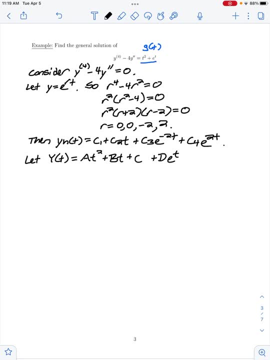 would be solutions of the homogeneous equation. so we need to take this quadratic that we started with and multiply by t squared, since 0 was a double root, And that would give us a t to the fourth, plus bt cubed, plus ct squared. 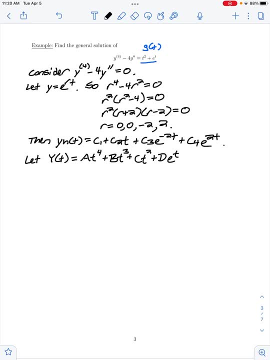 And then I have a constant times e to the t, which was not part of the whole equation, and then I have a constant times e to the t, which was not part of the whole equation, and then I have a constant times e to the t. 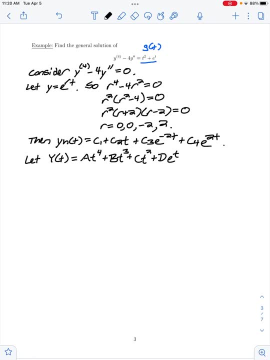 which was not part of the whole equation, so this should now be the correct form And to substitute this into our non-homogeneous equation. well, since it's a fourth order equation, we're going to need our first four derivatives. So for y prime. 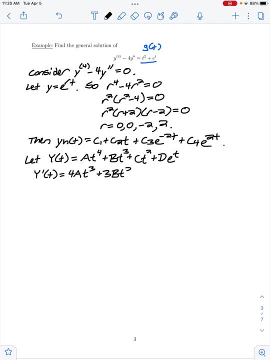 we would have 4a t cubed plus 2CT plus DE to the T. For the second derivative, we would have 12AT squared plus 6BT plus 2CT plus DE to the T. For the third derivative, we would have 24AT to the first. 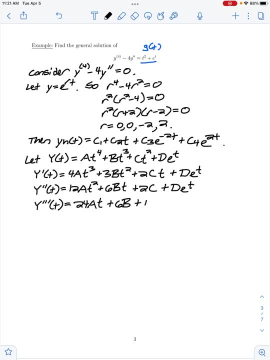 plus 6B plus DE to the T. And then, lastly, for the fourth derivative, we have 24A plus 24B plus DE to the T. So, taking these expressions and substituting into our non-homogeneous equation, we have the fourth derivative of y, which would be 24a plus d e to the t. 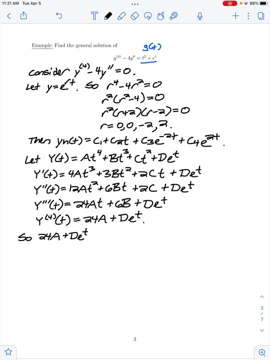 and then minus 4 times y double prime. So for negative 4 times y double prime we have a negative 48a t squared minus 24b t, minus 8c, minus 4d e to the t and we need this to equal our g of t function. 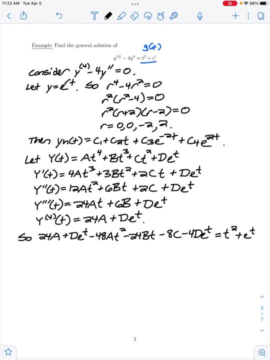 which was t squared plus e to the t. So collecting like terms, on the left-hand side we have a negative 48a t squared minus 24b times t, then a constant of 24a minus 8c and then minus 3d e to the t. 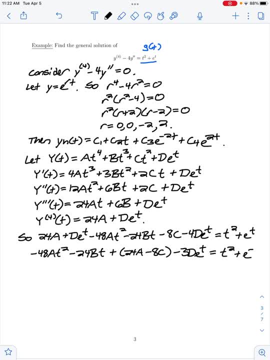 And this has to equal our t squared plus e to the t power. So when we equate these coefficients, starting with the t squared terms, we have negative 48a has to be 1.. So a is negative 1 over 48.. 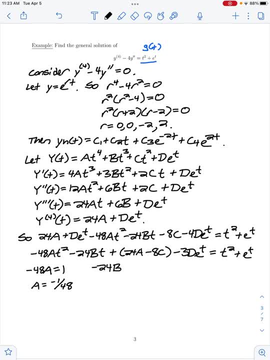 Negative 24b has to be 0. So therefore b is 0. Our constant term, 24a minus 8c, has to equal 0. So that means c is equal to 3 times a. So c would be negative 3 over 48.. 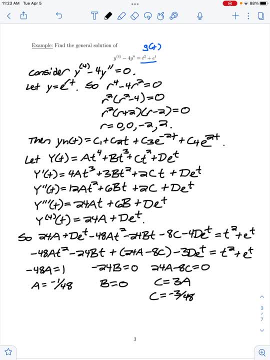 And then, lastly, equating the coefficient for the exponential, we have negative 3 over 48.. So that means c is equal to 3 times a, So negative 3d is 1.. So d is negative 1. third. 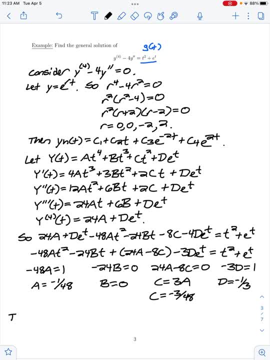 So let's see what we have for our particular solution y of t. We have a which is negative 1 over 48, t to the fourth power plus 0 t cubed, plus c, which is negative 3 over 48, t squared. 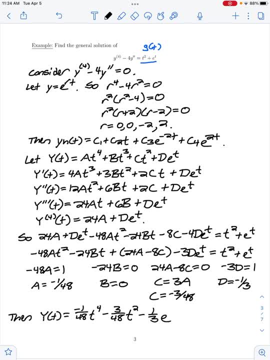 plus d, which was a negative 1 third e to the t. And so for our general solution of this non-homogeneous equation, we have our homogeneous solution: c1 plus c2t plus c3 e to the negative 2t. 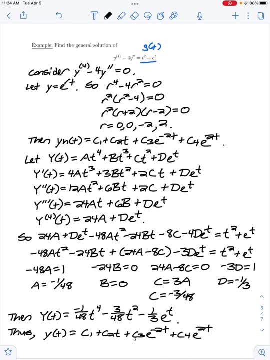 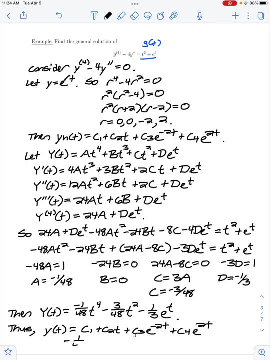 plus c4 e to the positive 2t. And then we add our particular solution, which was the negative 1 over 48, t to the fourth, minus 3 over 48, t, squared minus 1 third e to the t. 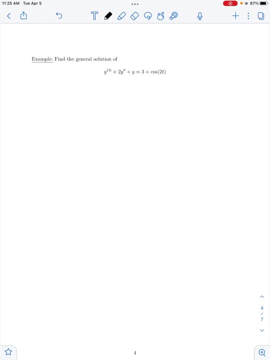 Okay, So let us consider some other examples. For our next one we have the same sort of question. We are asked to find the general solution of this fourth order linear, non-homogeneous equation with constant coefficients. So again, we will start by considering. 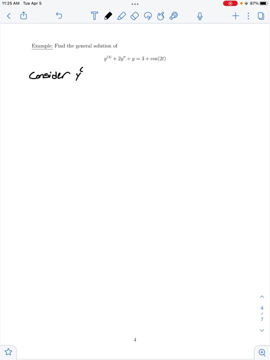 the corresponding homogeneous equation. So if we simplify this equation, The fourth derivative of Y plus 2Y, double prime plus Y equals 0.. And to solve this we look for solutions of the form: Y equals e to the rt power, which gives us a characteristics equation of R to the fourth plus two, r squared plus 1, t squared plus y, times two plus 1 minus four. 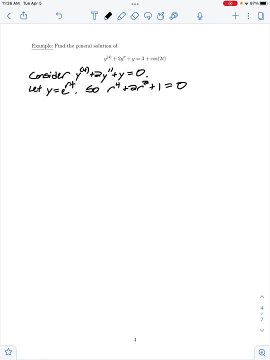 one is zero and this can be factored as r squared plus one quantity squared. so we find that our roots are plus or minus i with a multiplicity of two. so for these repeated, complex conjugate roots, our homogeneous solution would have the form: c1 cosine t plus c2 sine t. 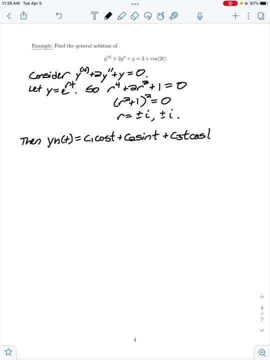 plus c3 times t, cosine t plus c4 t sine t. and now we need to find our particular solution. so again, to use the method of undetermined coefficients. we look at this g of t function on our right hand side and we see that it is the sum of a constant and a constant times cosine of 2 t. 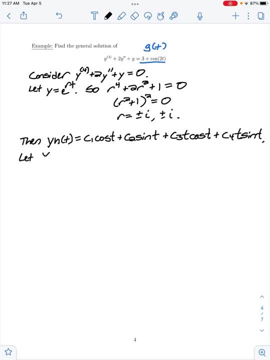 so for our particular solution, let us consider some of the same form, let's say a constant a plus, since we had a constant times cosine of 2t, i have to consider both a constant times that cosine function and another constant times that sine function in comparing this with the homogeneous solution. 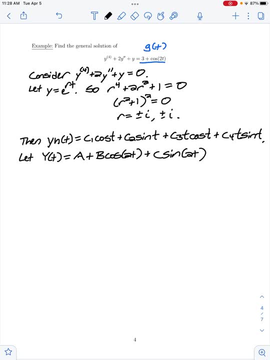 we see that none of these terms are already part of the homogeneous solution, so this should be the correct form for our particular solution. now, to substitute this into our non-homogeneous equation, since it's fourth order again, we need to find our first four derivatives. so, starting with y prime, we would have a negative 2b. 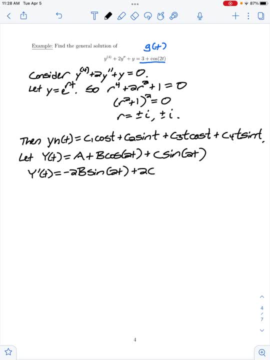 sine of 2t plus 2c cosine of 2t. then for the second derivative we would have negative 4b cosine of 2t minus 4c sine of 2t. for the third derivative we would have a positive 8b sine of 2t. 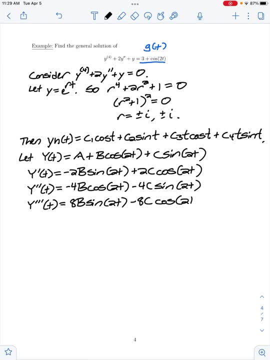 minus 8c cosine of 2t. and then, lastly, for the fourth derivative, we have 16b cosine of 2t and plus 16c sine of 2t. So substituting these expressions into our non-homogeneous equation we're looking for. 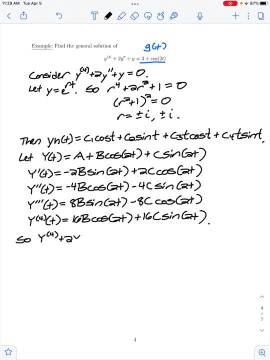 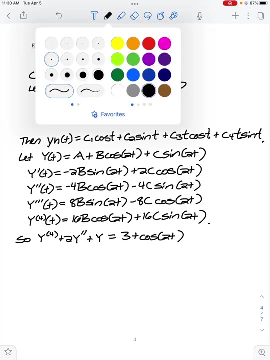 the fourth derivative plus 2 times y, double prime plus y, and that needs to equal our g of t, function 3 plus cosine of 2t. And so let's see what we have when we substitute these terms into the left-hand side and collect like terms. So I'm looking at my fourth derivative. 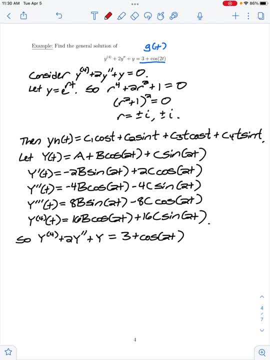 the second derivative and the original function. So let's group the sine and cosine of 2t terms together. So, starting with the sine terms for y, the fourth derivative, plus 2 times y, double prime plus y, we are left with a total of 9c. sine of 2t. 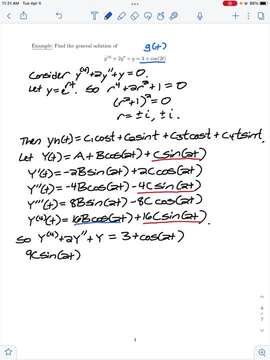 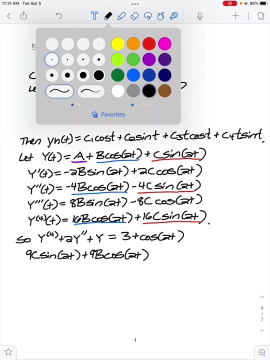 Then grouping my cosine of 2t terms for the fourth derivative plus 2 times the second derivative plus y, we have a total of 9b cosine of 2t. And then, lastly, I have this constant term for y. 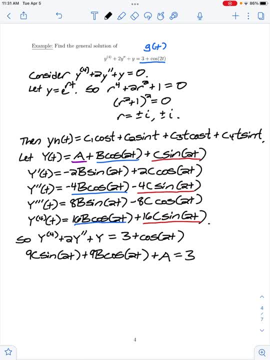 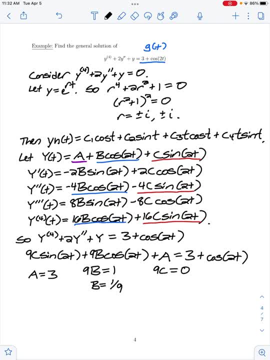 And equating the sine coefficients, we see 9c has to be 0, and therefore c is 0.. So this means that our particular solution, capital Y, is given by a, which was 3,, plus b, which was a, 1, ninth cosine of 2t, and then plus a, 0, sine of 2t. 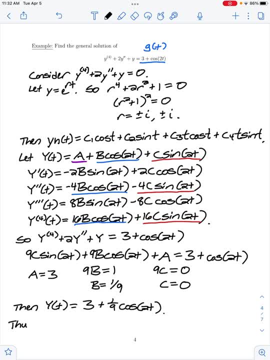 And so, finally, our general solution of this non-homogeneous equation is the sum of our homogeneous solution: c1 cosine t plus c2 sine t plus c3 t cosine t plus c4 t sine t, plus our particular solution: 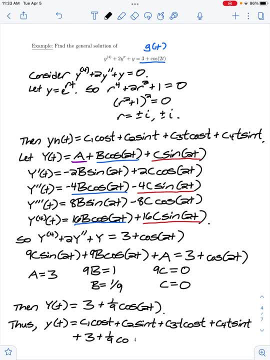 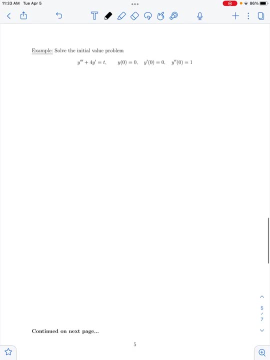 which was 3, plus 1 ninth cosine of 2t. So let's now consider an example of a non-homogeneous higher order equation paired with a set of initial conditions. So here we are asked to solve this initial value problem. 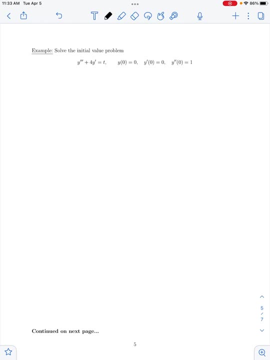 where we have a third-order non-homogeneous linear equation with constant coefficients and we have three initial conditions involving y, y prime or y double prime at time 0.. So, again for a non-homogeneous equation, our first step is to consider the corresponding homogeneous. 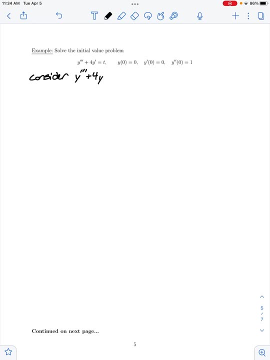 equation y, triple prime plus 4y prime equals 0.. And to solve this we could look for solutions of the form: y equals e to the rt power, so that r is a root of the characteristic equation. r cubed plus 4r is 0.. 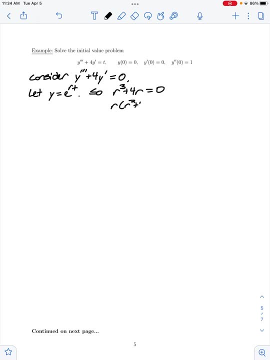 So factoring out an r leaves me with r. squared plus 4 is 0. And so I find that my roots are 0, or plus or minus 2i. So my homogeneous solution has the form c1 plus c2, cosine t. 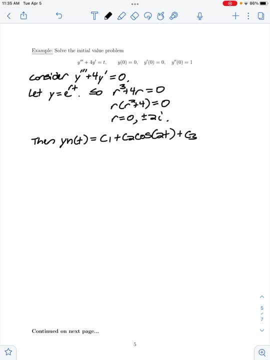 sine of 2t plus c3 sine of 2t. And now we need to find a particular solution of our non-homogeneous equation. And when I look at my g of t function on the right-hand side, I see that it's just t or a first-degree polynomial. 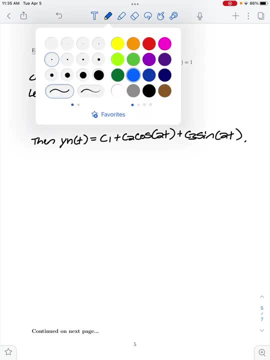 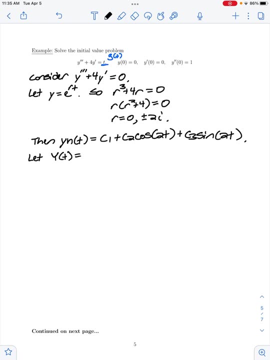 or a linear. So we could consider a particular solution, capital Y- of that same general form, a linear polynomial, something like at plus b. But we see that since 0 was a root of our characteristic equation, a constant is already part of the homogeneous solution. 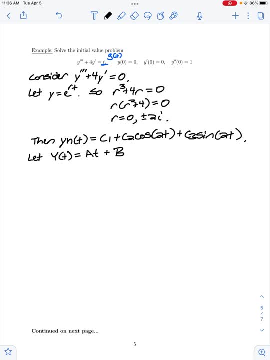 So we need to take our first-degree polynomial for the particular solution and multiply by t to the first power, giving us At squared plus Bt. And now none of these terms are part of our homogeneous solution. So from here we need to find our first three derivatives to substitute into: 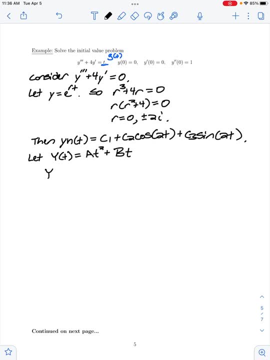 non-homogeneous equation and we find that our first derivative would be 2a, t plus B. our second derivative is 2a and so the third derivative is 0, so substituting into our non-homogeneous equation, we're looking at y, triple prime. 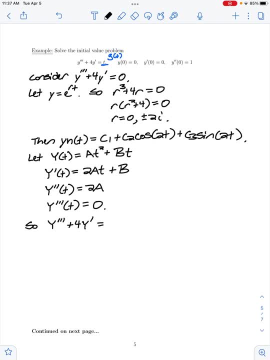 plus 4y prime, which needs to equal G of T, and so substituting these expressions in well, y triple prime was 0. so we just have 4 times y prime, which would be 8, a, T, 4b, and this needs to be equal to T. so equating our coefficients, we find 8a has to be 1. so 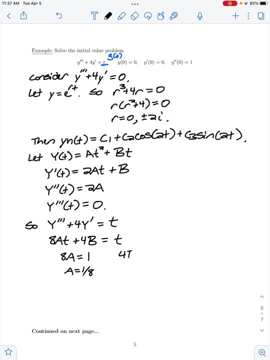 a is 1 eighth and 4b has to equal 0, so b is 0, and so we find that our particular solution, capital Y, is equal to a, which was 1 eighth T squared plus 0 T. so our general solution Y of T for this non-homogeneous equation would be our homogeneous. 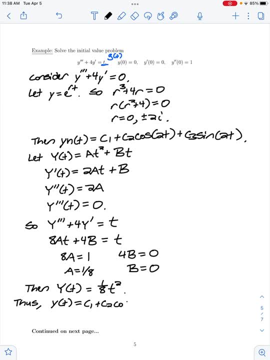 solution: C 1 plus C 2, cosine of 2 T plus C 3 sine of 2 T, plus my particular solution, which was 1: 8 T squared. so now to finish out the problem I need to solve for my constants by making use of: 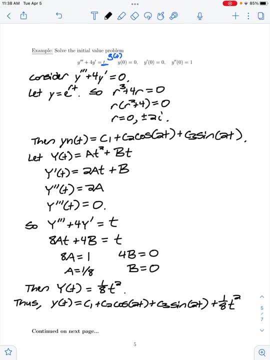 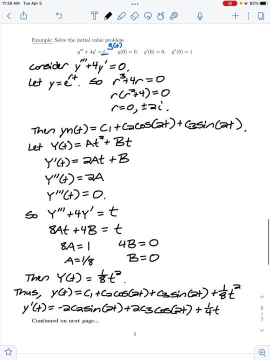 the initial conditions, which means that I need to find my first and second derivatives of this general solution. so let's take a look at y prime here. for y prime we would have negative 2 C, 2 sine of 2 T plus 2 C, 3 cosine of 2 T plus 2 eighths, or 1, 4 T, and then for my 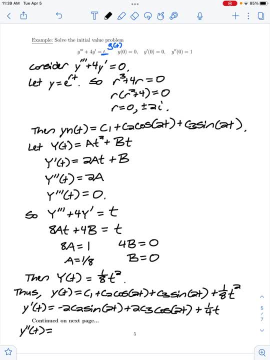 second derivative y double prime, we would have negative 2 C 2 sine of 2 T plus 2 C 3 cosine of 2 T plus 2 eighths or one-fourth T. and then for my second derivative y double prime, I would have a negative 4C2 cosine of 2T plus, excuse me, minus 4C3 sine of 2T plus one-fourth. 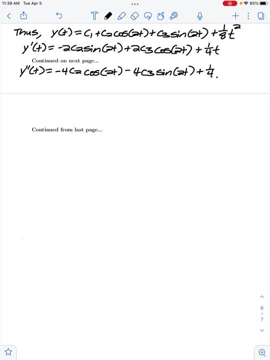 So let's now apply our initial conditions. Looking at Y at 0, we're left with C1 plus C2, which we were told must be 0. Y prime at T equals 0 gives us 2C3,, which we were told must be equal to. 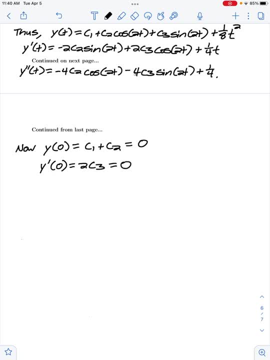 2C3.. And then, lastly, for our second derivative, Y double prime at T equals 0, we're left with a negative 4C2 plus one-fourth, which we were told must be equal to 1.. So let's see what this gives us. 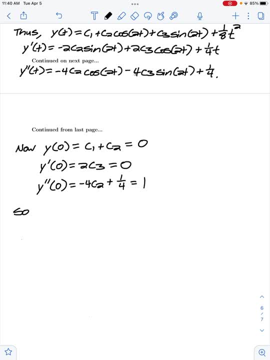 Okay, Looking at my third equation I could solve for C2.. I find that negative 4C2 is equal to 1 minus one-fourth, so three-fourths. And then, dividing through by negative 4,, we find C2 is negative three-sixteenths. 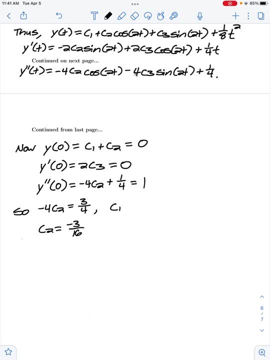 From looking at my first equation, I could solve for C1 in terms of C2.. C1 has to be the negative of C2, so that would be a positive three-sixteenths, And from the second equation it follows immediately that C3 is 0.. 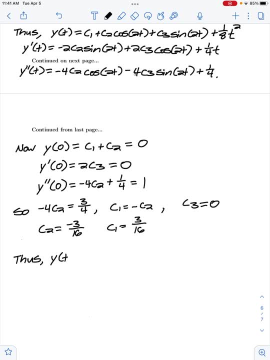 So our solution of this initial value problem would be C1,, which was three-sixteenths, plus C2,, which is negative three-sixteenths times cosine of 2T, plus C3,, which was 0, sine 2T, and then plus my particular solution, which was a one-eighth T squared. 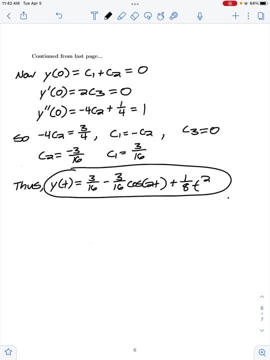 So here we have the solution of that initial value problem. So here we have the solution of that initial value problem which was 0, sine 2T, and then plus my particular solution, which was a one-eighth T squared. So here we have the solution of that initial value problem. 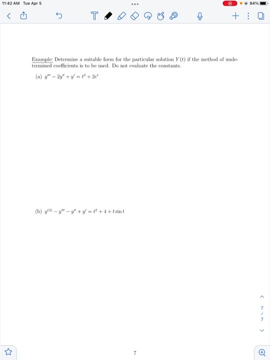 So for our last couple of examples in this section, let us consider some examples of finding the correct form for a particular solution if we're using the method of undetermined coefficients. So here we are, asked to find the correct form of our particular solution. 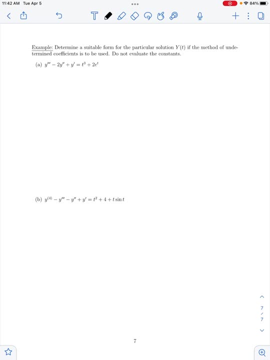 but do not evaluate the constants, Don't worry about solving for the coefficients. So for part A of this example, we have a third-order linear, non-homogeneous equation with constant coefficients. And so we start by considering the homogeneous equation: y, triple prime minus 2y, double prime plus y prime is 0.. 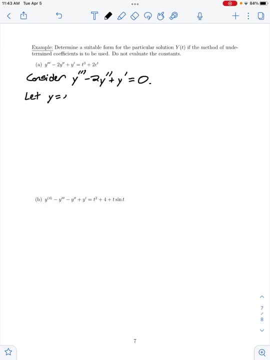 In looking for solutions of the form y equals e to the rt, we obtain a characteristic equation of r, cubed minus 2r, squared plus r, equals 0.. So, factoring out an r, I am left with r squared minus 2r plus 1.. 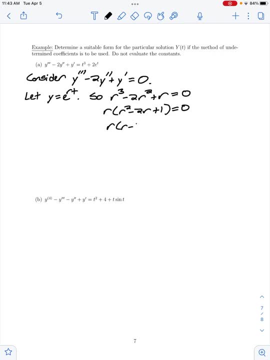 And that can be factored as r minus 1, quantity squared. So I find that my roots would be 0 and 1, which has multiplicity 2.. So here our homogeneous solution would be of the form: c1 plus c2, e to the rt. 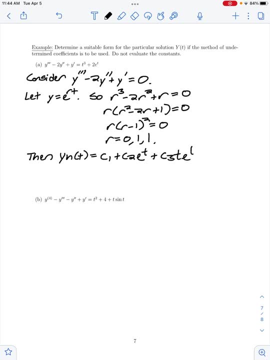 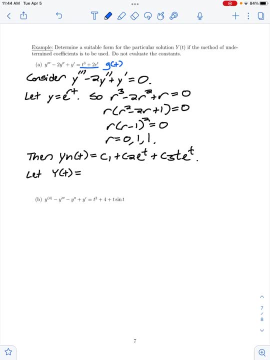 So here g of t is a cubic or a third-degree polynomial Plus a constant times e to the t. So we might start by considering a general cubic at cubed plus bt, squared plus ct plus d, And then add a constant times e to the t power. 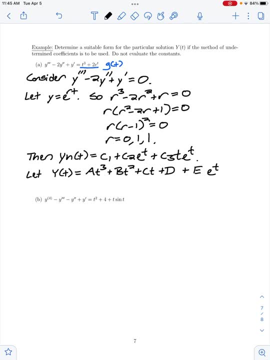 Now, when we compare these terms with our homogeneous solution, we see that, since 0 was a root of the characteristic equation, one of the terms in our homogeneous solution is a constant, So we need to take our third-degree polynomial, which involved a constant d on the end. 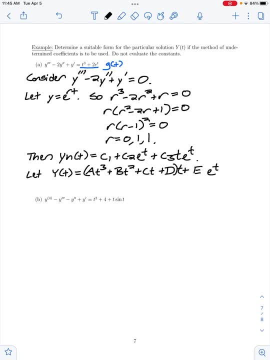 and multiply by t to the first power And then we had r equals 1 was a double root of the characteristic equation. So our homogeneous solution also contains a constant times e to the t and a constant times t e to the t. So our last term for the particular solution where we have a constant times e to the t, 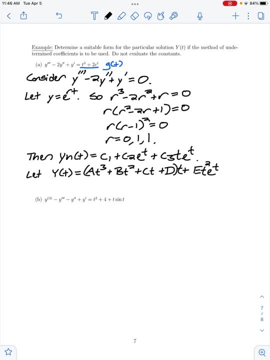 must be multiplied by t squared, since 1 was a constant times e to the t And 1 was a double root. So this gives us a particular solution of the form at to the fourth, plus bt cubed, plus ct squared plus dt plus e times t squared e to the t. 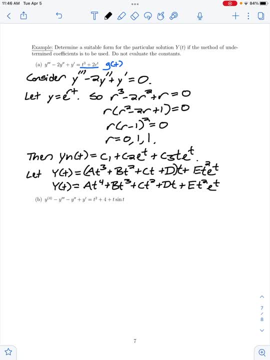 And so let's look Next at part b. in part b we have a fourth-order linear, non-homogeneous equation with constant coefficients. So same approach. to begin with We can consider the homogeneous equation the fourth derivative of y minus y triple prime. minus y double prime, plus y prime. 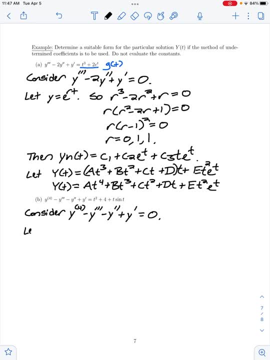 is equal to 0.. And if we're looking for solutions of the form e to the rt, then we obtain a characteristic equation of r to the fourth, minus r, cubed, minus r squared, plus r is equal to 0.. And to solve this I could factor by grouping some: 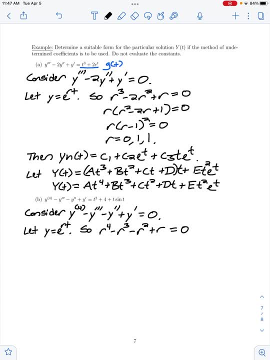 common terms together. From my first two terms I could factor out an r squared, which would leave me with r squared minus r, And then, from the last two terms, if I factor out a negative, I'm left with r squared minus r. 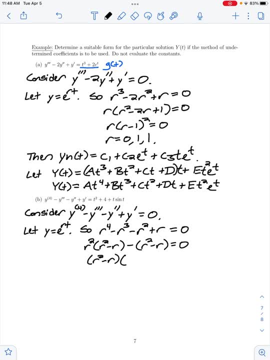 So, factoring out a common r squared minus r, I'm left with r squared minus r, So factoring out a common r squared minus 1.. And then, if I factor an r from the first of these factors, I'm left with an r minus 1.. 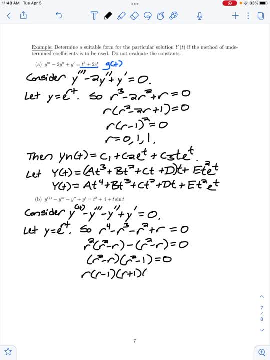 And then, factoring my r squared plus 1,, I have an r plus 1 times r minus 1.. And so I find that I have roots of 0, negative 1, and 1,, where 1 has multiplicity of 2.. 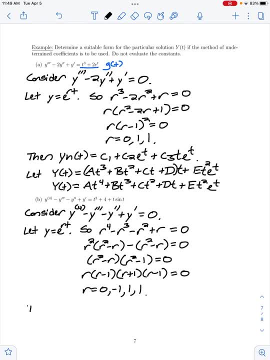 It was repeated. So for my homogeneous solution I have c1 plus c2 times e to the negative t, plus c3 e to the t plus c4, plus c3 e to the t. And now let's consider our particular solution. 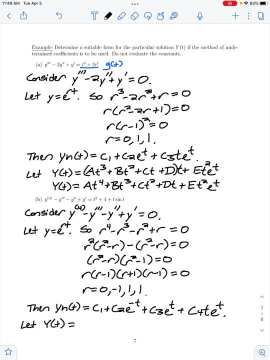 capital Y. So to determine the form of our particular solution, we're going to look at the form of this g of t function on the right-hand side And we see that the first two terms are a quadratic polynomial or a second degree. 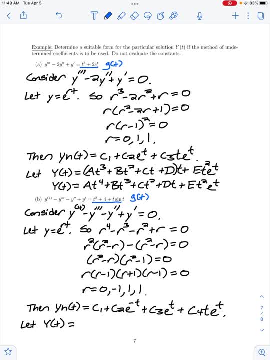 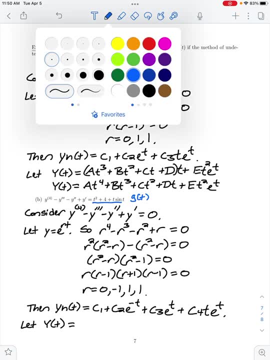 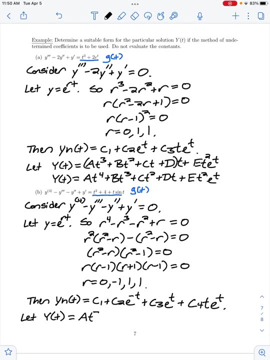 and then plus I have a linear term or a first degree polynomial times sine of t. So for our particular solution we might start with the same general form. Let's take a general quadratic at squared plus bt, plus c, And then we could add a linear term.